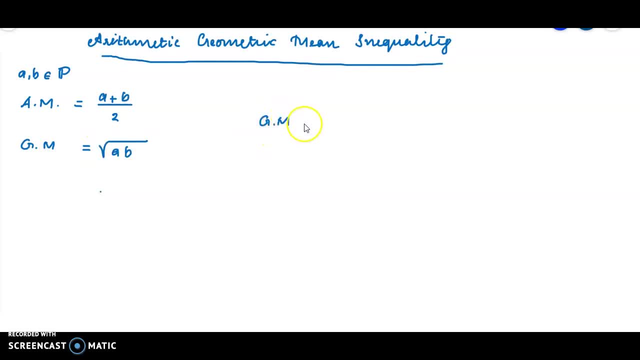 Geometric mean is less than or equal to arithmetic mean, For we extend it to n real numbers, It should be positive Geometric mean less than or equal to arithmetic mean If we have two real numbers: Root of a, b, less than or equal to a plus b divided by 2.. 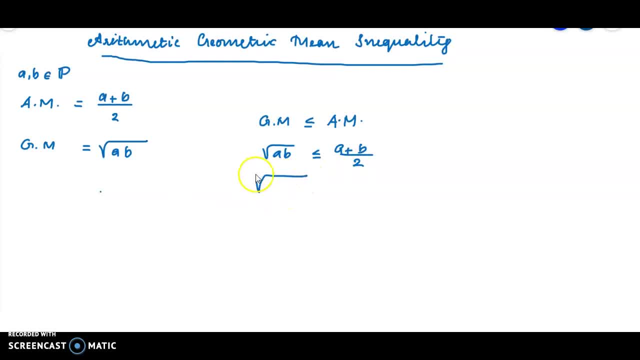 If we have n, three real numbers, Root of a, cube, root of a into b, into c, Less than or equal to a plus b plus c divided by 3. And we can extend the result to n real numbers, n, the root of a, 1 into n numbers, etc. 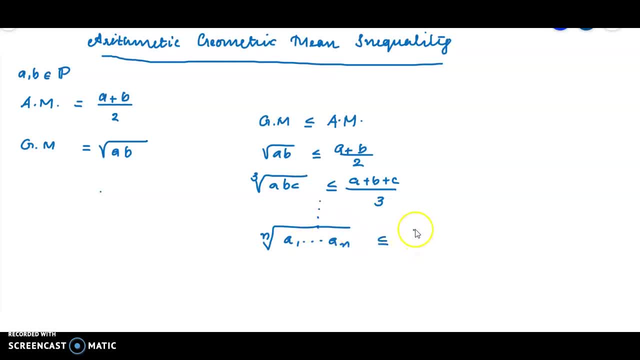 a n less than or equal to, then the arithmetic mean a 1 plus etc. plus a n divided by whole, divided by n, And this can be written as a 1, a, 2, etc. a n product n. the root is denoted by the power 1 by n, less than or equal to 1 by n, into a 1 plus a 2 plus etc. plus a n. 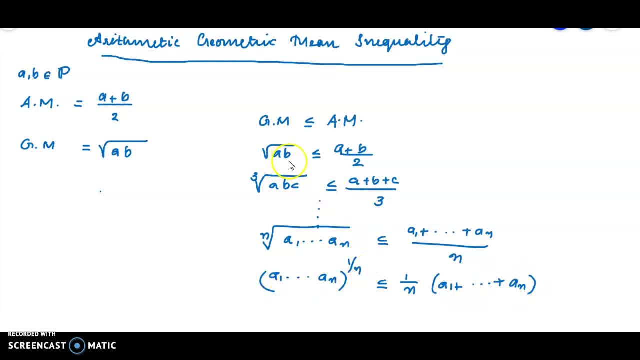 So the relation of 1 by n is raised to 1 by n. Here a b raised to 1 by 2, less than or equal to a plus b divided by 1 by 2 of a plus b. This is not written like that. 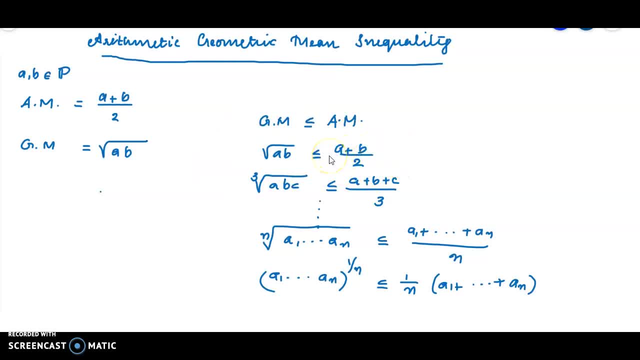 But since this is simple, we write root a b equal to a plus b divided by 2.. Given two positive real numbers, arithmetic mean is the sum Given two, or any sum divided by number of numbers. Geometric mean is the if there are n numbers. 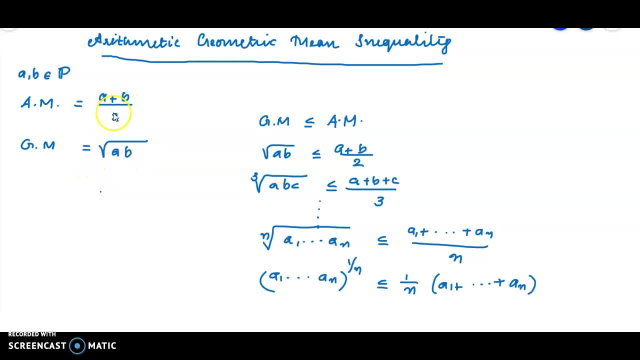 And the root of the product of the numbers. If there are two numbers, 1 by 2, a plus b- arithmetic mean and root of a, b geometric mean- That is about arithmetic mean and geometric mean- Then we can move to the proof of the inequality. 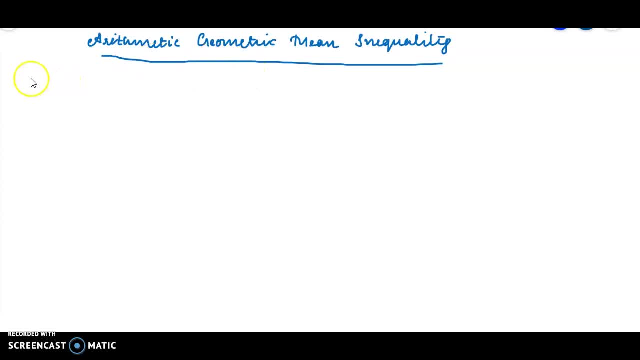 Now we move to the statement of arithmetic geometric mean inequality. The inequality states that the statement is like this: Root of a, b, less than or equal to 1 by 2 of a plus b. 1 by 2 of a plus b. 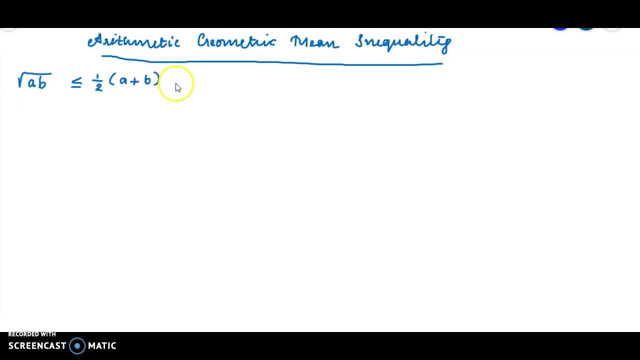 A little better: a: b raised to 1.. 1 by 2 of a plus b. Root of b raised to 1.. 1 by 2 of a plus b. But we write 2 by 2, like this For all positive real numbers a and b. 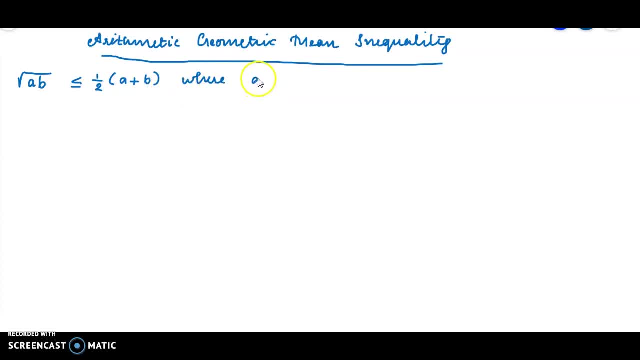 Where statement completes: Where a, b are positive, positive real numbers, b elements. b elements are not 0.. positive none can be 0.. positive element of b positive real numbers: 0.. one number is not 0.. 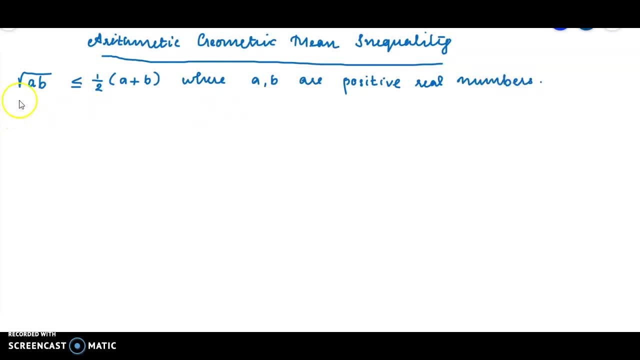 both are positive. real numbers are number. geometric mean less than or equal to minus, like a gm, less than or equal to a m. and I'm gonna run it. you know, I'm gonna proof like a boa. I'm gonna make another. hey, be positive on a comma. be greater than zero. 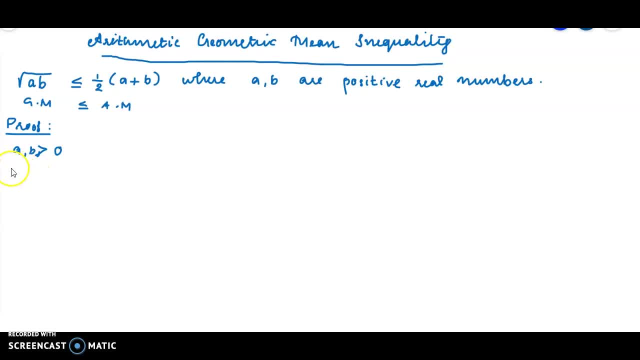 and I'm gonna turn it. you know, I'm gonna put a little touch a root, a root. be positive. a root a root, b greater than zero. now assume that a naught equal to B, assuming a naught equal to B, a and B equal ala. 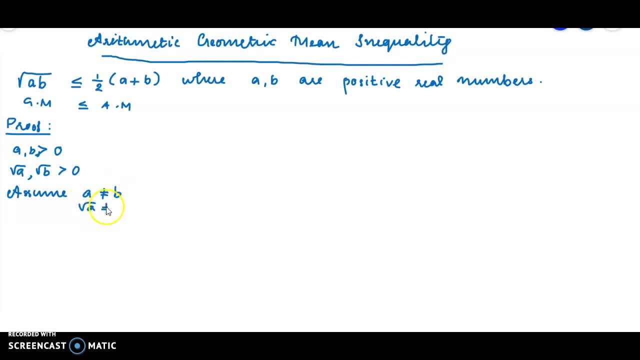 and clic-a-dick a route a not equal to root B in Nauruga, parent static in place root and on tickle to Ruby. now you consider the difference root a minus Ruby, equal. ala our differences. a Roth in Allan, America morning and the square. 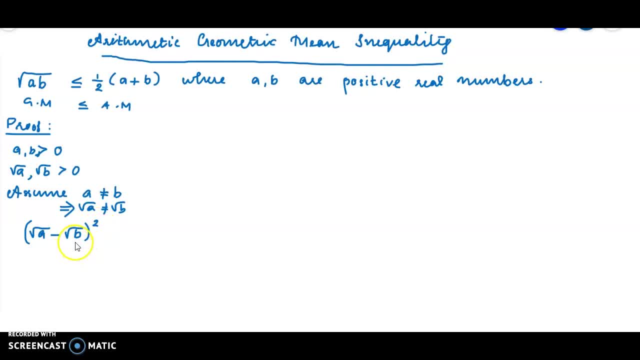 root a minus root b. square difference. is it positive or negative? it is not 0. root a and root b are not equal, but if we take square it will be positive, strictly greater than 0. under the assumption a not equal to b, we can write root a minus root b. 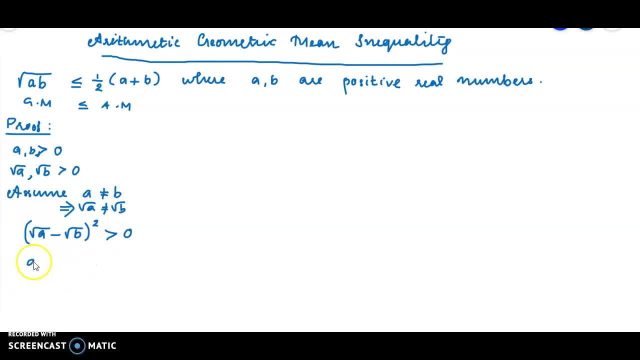 whole square is greater than 0, then square a, then a minus 2 product root a into root b. I can write it as root of ab plus root b to square this is greater than 0. or you can write: a plus b is strictly greater than 2. root of. 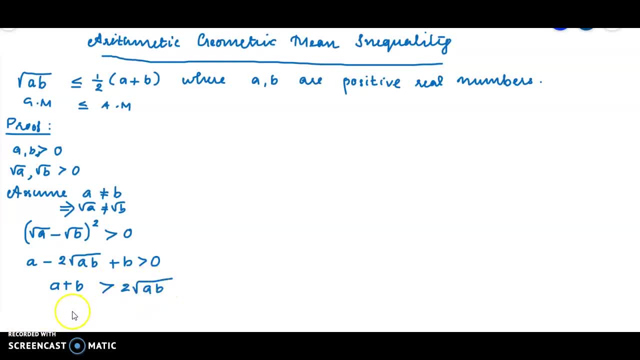 ab. then you can write: a plus b divided by 2 is greater than root of ab, which implies rate the inequality in reverse order: root ab less than root ab. less than half of a plus b. root ab less than half of a plus b. so when does strict less than come? 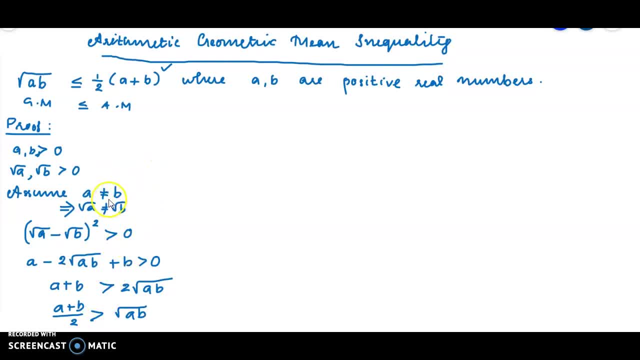 if the numbers are not equal, if a and b are unequal, then we get the strict inequality root ab: less than half of a plus b. when it is equal, then the possibility is less than half of a plus b. so when it is equal, then we have got. 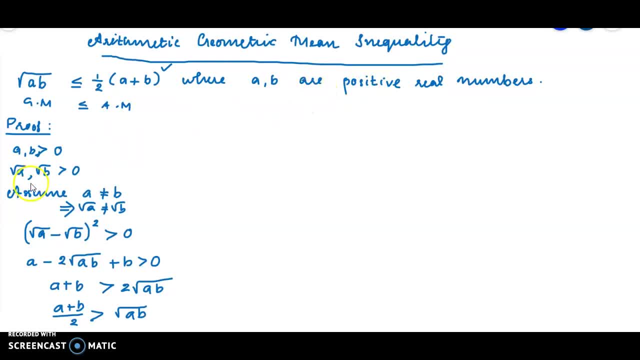 poitmaker, we have not shown that expressions. also, we already know that that room another case on case of enough us R less or become okay, ok, excuse me, not up only the script in quality. roosten only won't be in c, it not only will move. 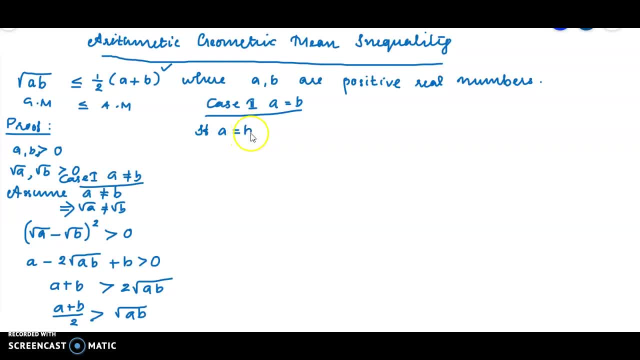 me, sea against me. If a is equal to b, then what will be the arithmetic mean? Arithmetic mean is equal to sum of the two numbers a plus a divided by 2.. That is 2a divided by 2.. That is a. 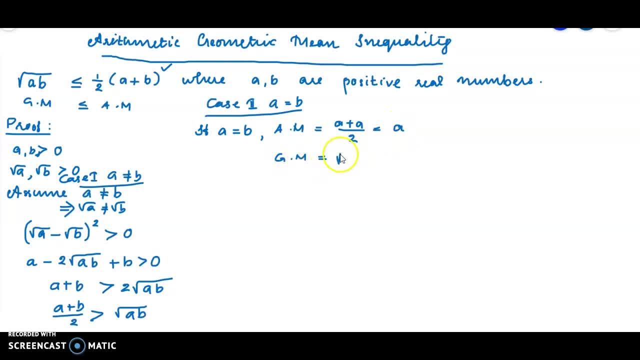 Then geometric mean is equal to root of a b, Root of a into a, a into a a. square root is equal to a. That means a m equal to g m, a m equal to g m or root of g m equal to a m. 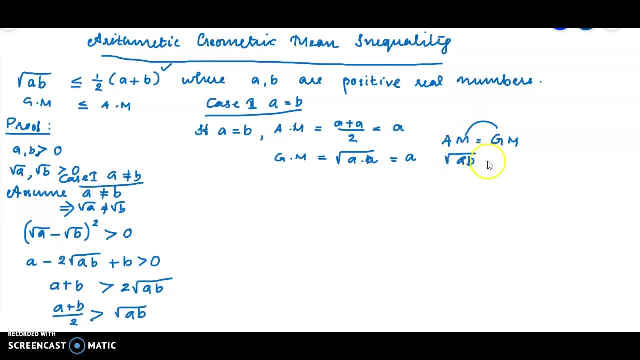 Then root of a- b equal to root of a, b equal to half of a plus b. Half of a plus b. if a equal to b, a m equal to b. If a equal to b, Root of a- b equal to equality- False. 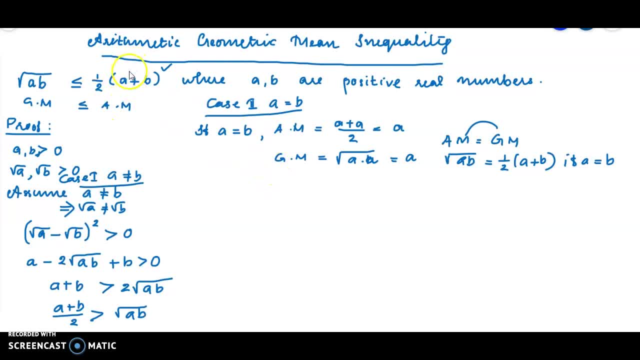 That means it is not true Now. it is only at this time that it is equal. If a and b are not equal, then we proved that it is Now. these two sides also proved that if a and b are not equal, then root of a b less than a plus b divided by 2.. 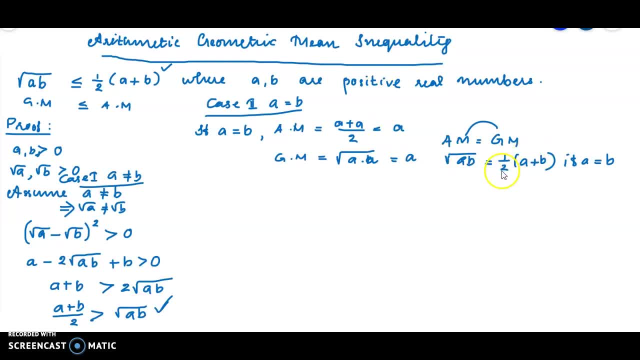 If a and b are equal, then root of a, b equal to half of a plus b. Root of a equal to half of a plus b is only when a and b are equal. We can prove the converse of this. Conversely, if g, m equal to a. 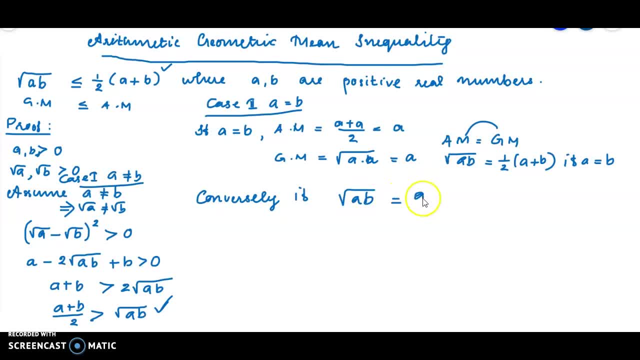 Root of a b equal to a plus b divided by 2.. Root of a b equal to a plus b divided by 2.. So what will happen? 2 into root of a b equal to a plus b, If we square that 4 a b equal to a plus b, whole square. 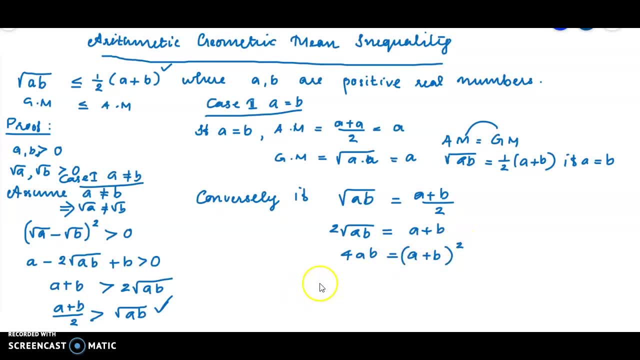 4 a b equal to a plus b whole square Or a plus b whole square. minus 4 a b equal to 0.. a plus b whole square is 2 a, b, a square and b square are not added, Then minus 4 a b comes to be a minus b whole square. 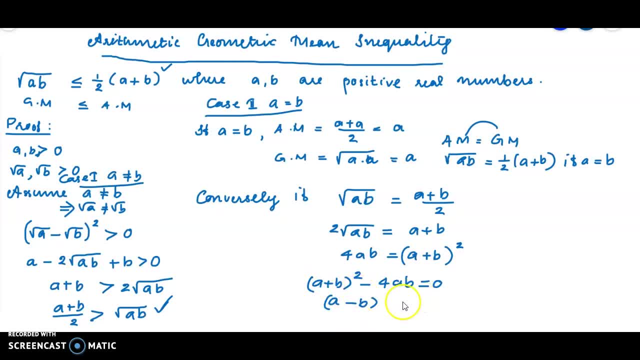 It is not explained. a square plus b, square plus 2 a, b minus 4 a b, That is a square plus b, square minus 2 a b. a minus b, whole square equal to 0. that in place, in place. in place a equal to be, a a minus b equal to. 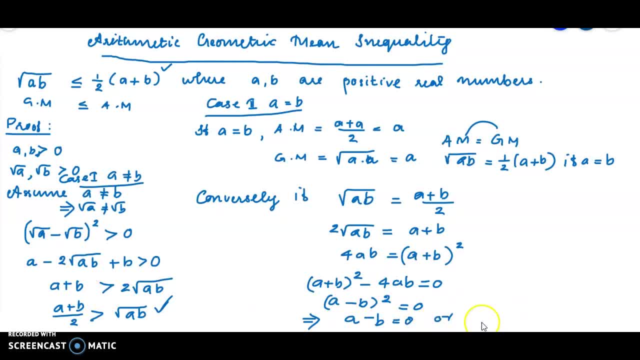 0 or a equal to b. square is a running numbers around: a minus b. 0 on a, equal to be a quality, met another 11, a equal to be a vehicle. on the matrona equality with a root a be less than that is root a be is less than a plus B divided by 2. 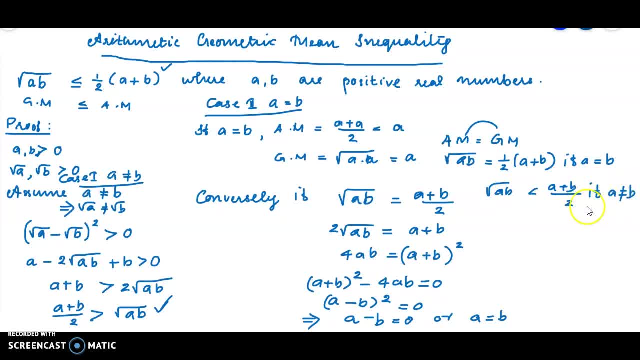 if a not equal to be, my case on and root a be equal to a plus B divided by 2. if I know, if I finally a equal to be, equal to be on with us. I'm working. it is emotional. a equal to be in another or upon a you don't know, any of you know. 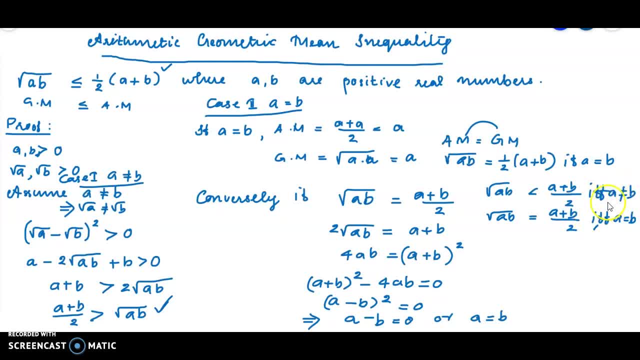 what you're less a little la n or you don't know any of. you know what you're less a little la n or you don't. equal to be on if an only a not equal to be, that is arithmetic mean, geometric mean. arithmetic. geometric mean inequality and we can extend the result.